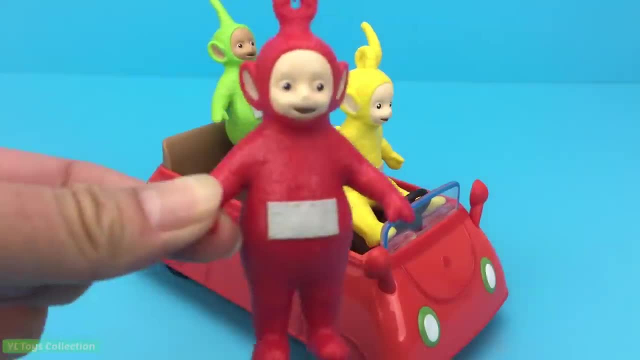 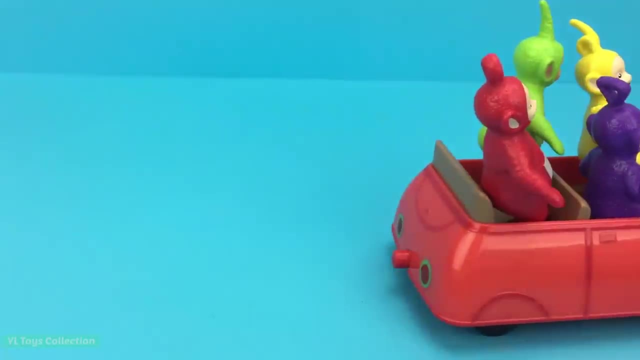 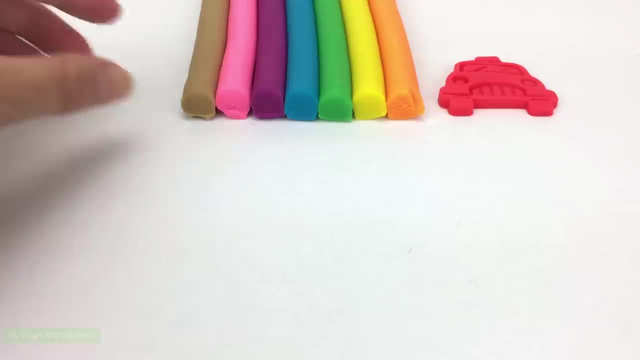 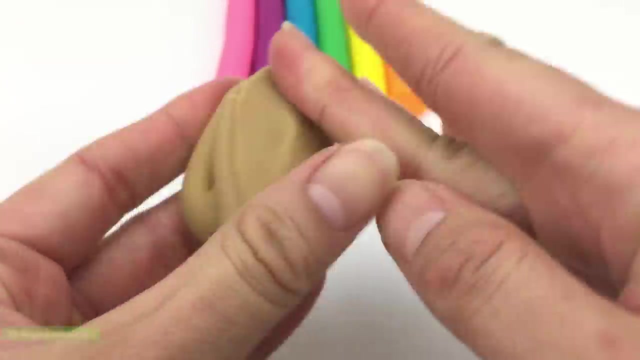 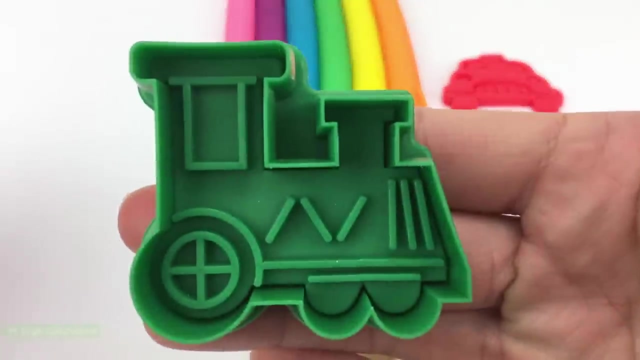 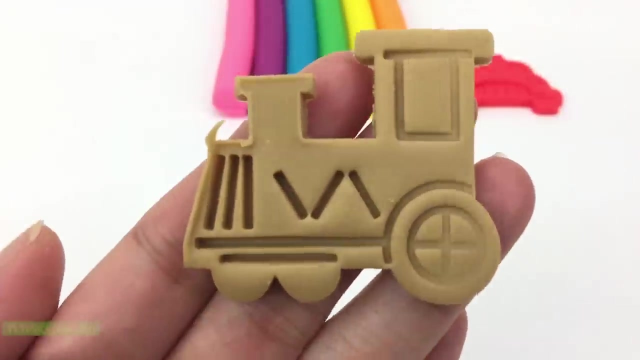 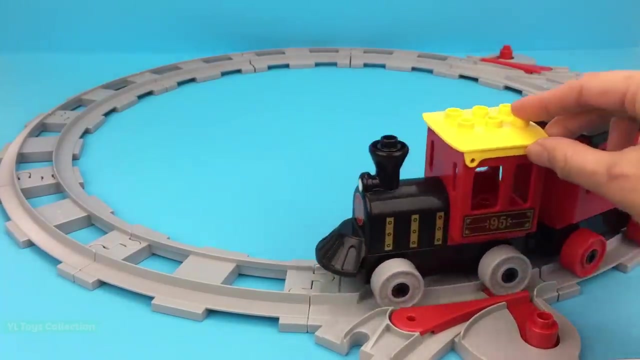 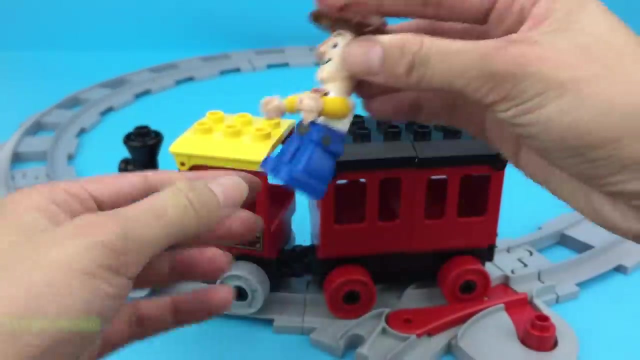 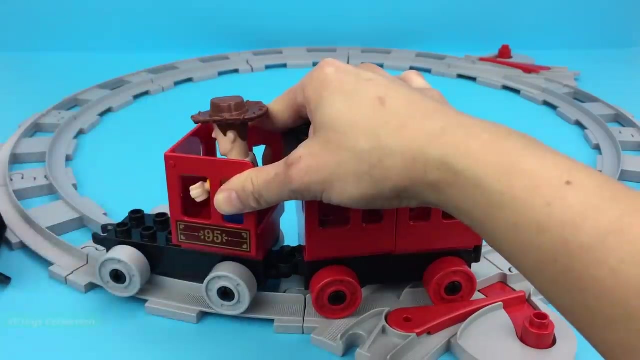 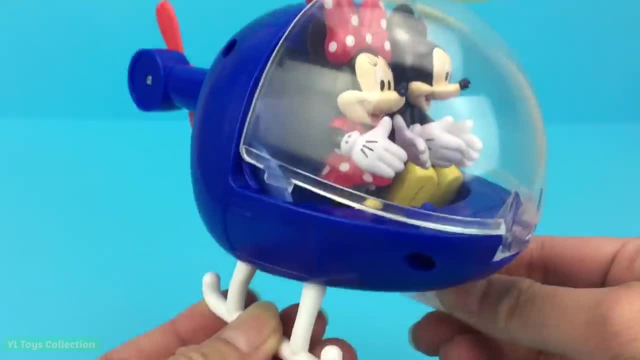 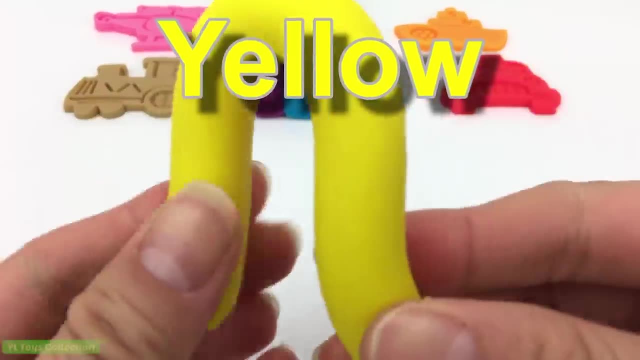 1,, 2,, 3,, 4,, 7, 8. 1,, 2,, 3,, 4,, 7, 8. Yellow Hickory, dickory dock. The mouse ran up the clock. The clocks don't run. 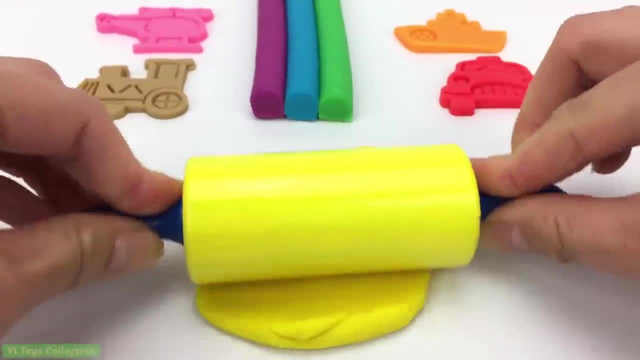 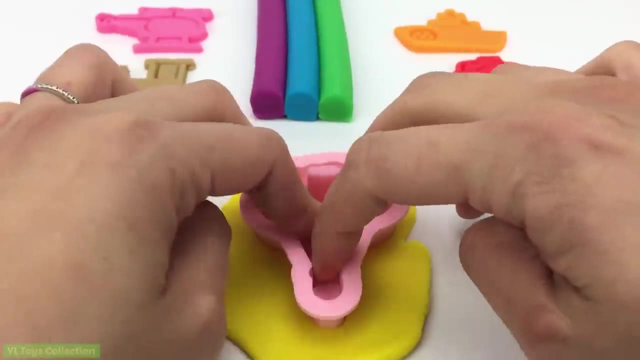 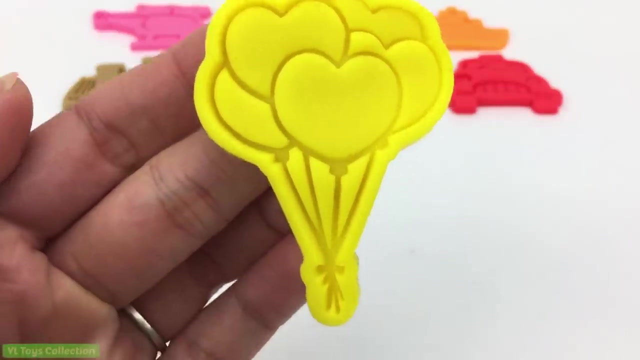 The mouse ran down. Hickory dickory dock, Tick tock, tick tock. Hickory dickory dock. the bird looked at the clock. the clock struck two away. she flew. hickory dickory dock, tick tock, tick tock. 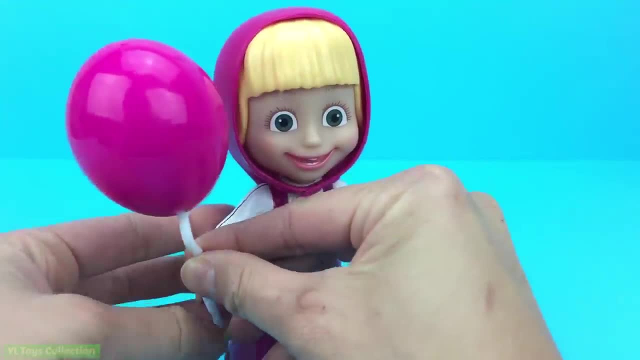 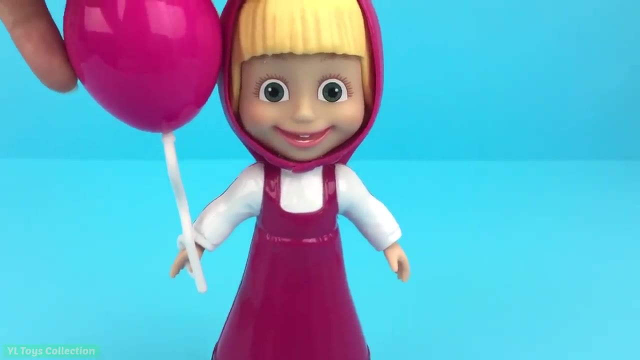 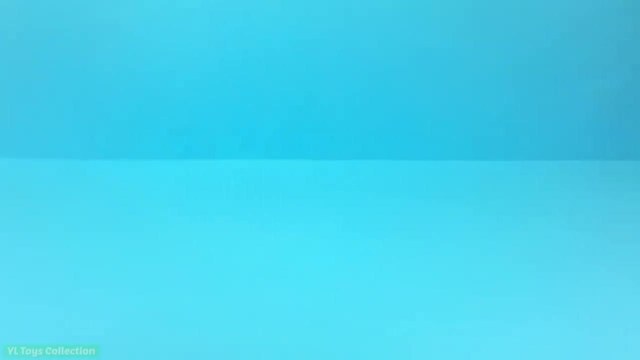 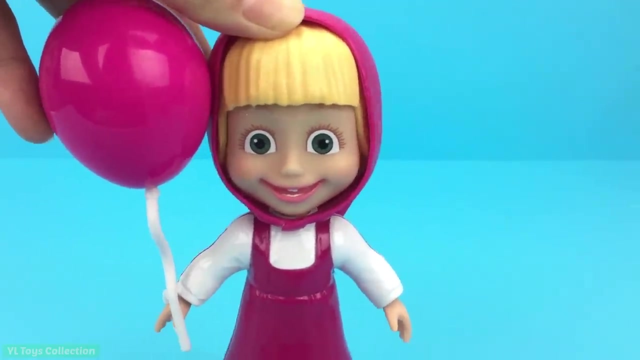 Hickory dickory dock. the dog barked at the clock. the clock struck three. it'll be three. hickory dickory dock. Hickory dickory dock. the bird looked at the clock. the clock struck two away. she flew. hickory dickory dock. 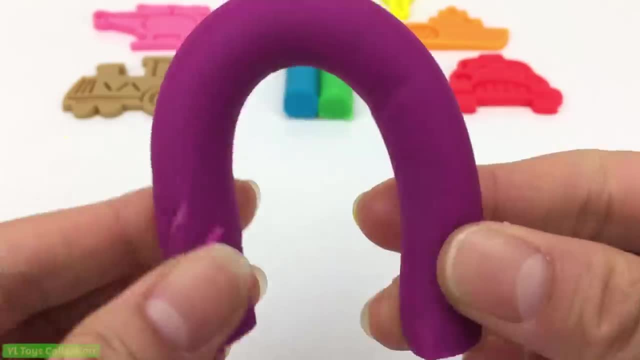 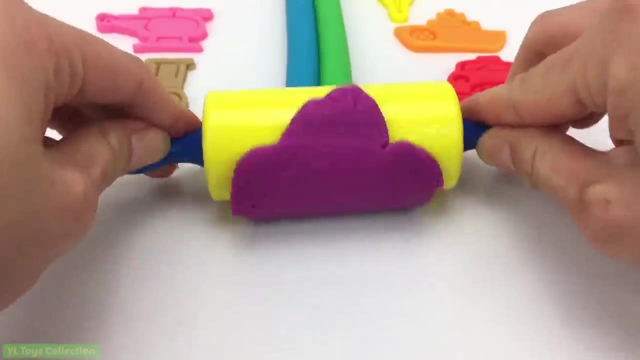 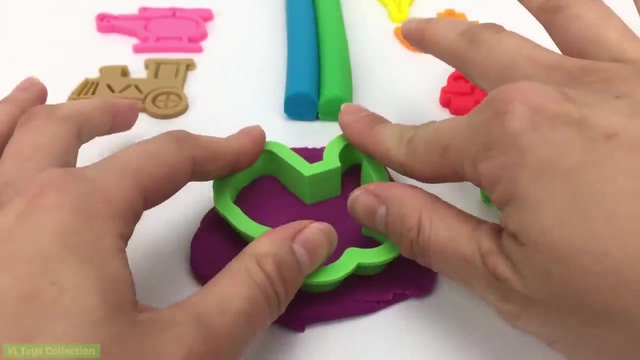 Purple Hickory dickory dock. the bee buzzed round the clock. the clock struck three. it'll be three. hickory dickory dock. The clock struck five. she went to her hide. hickory dickory dock, tick tock, tick tock. 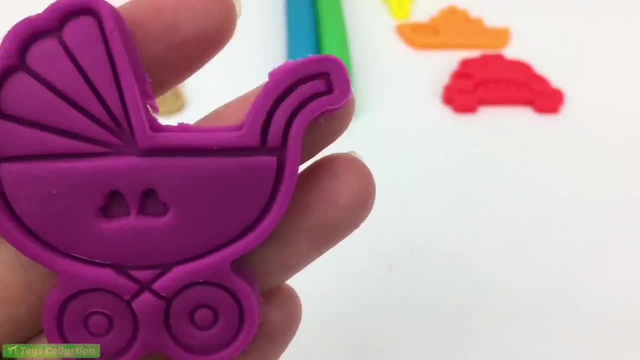 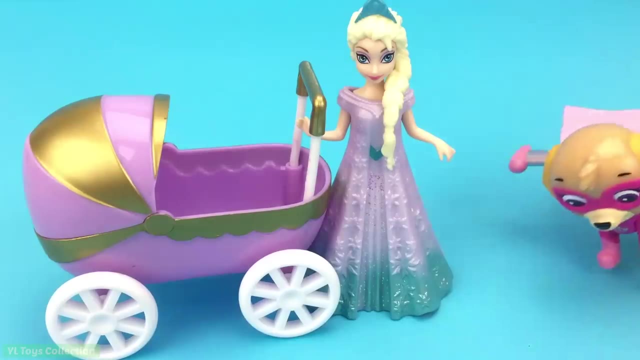 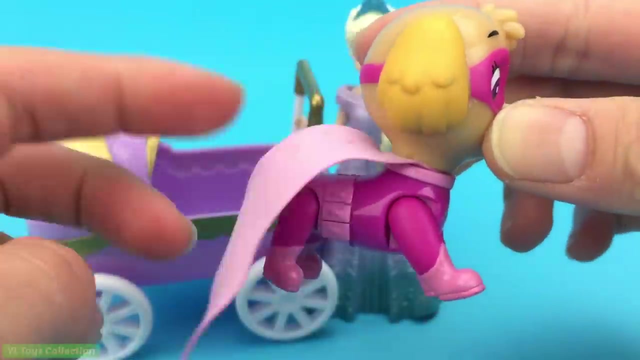 Hickory dickory dock. the bird looked at the clock. the clock struck six little six. hickory dickory dock, tick tock, tick tock. Hickory dickory dock, tick tock, tick tock. Hickory dickory dock, tick tock, tick tock. 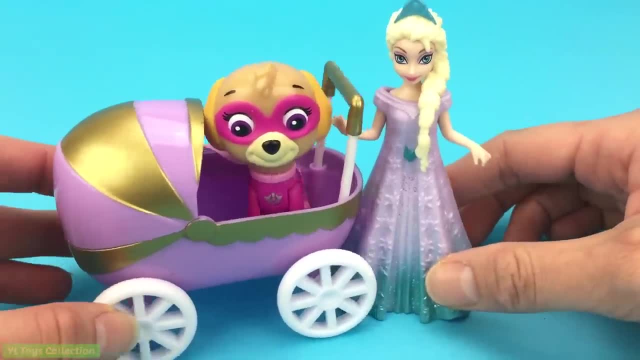 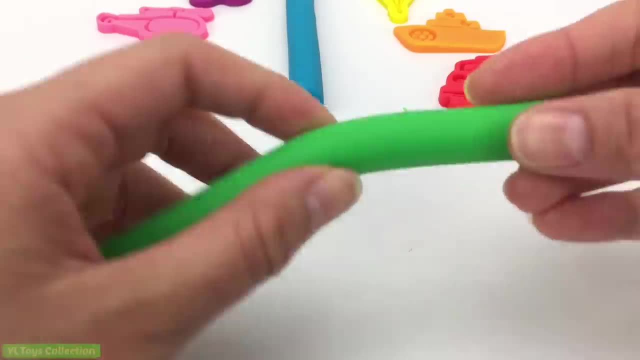 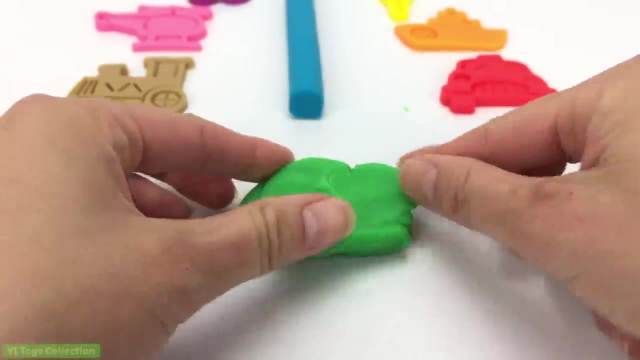 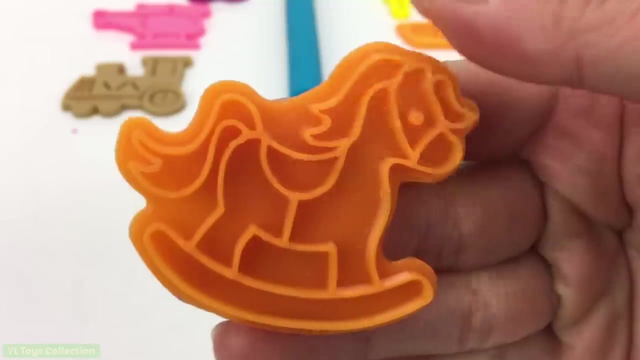 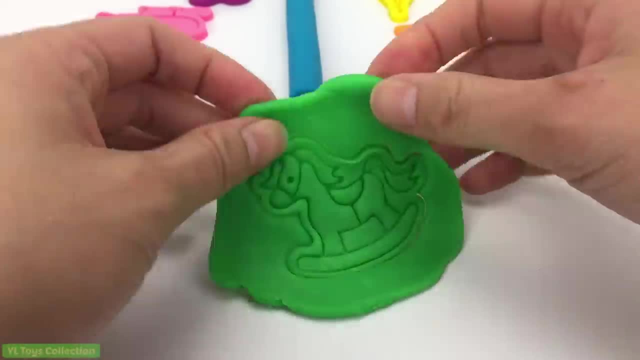 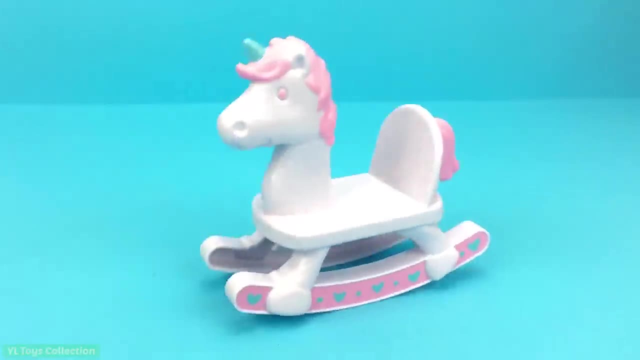 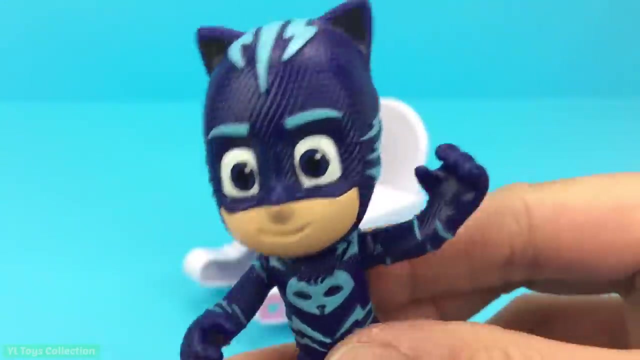 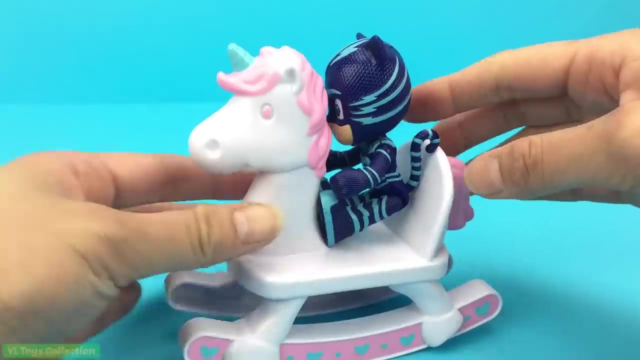 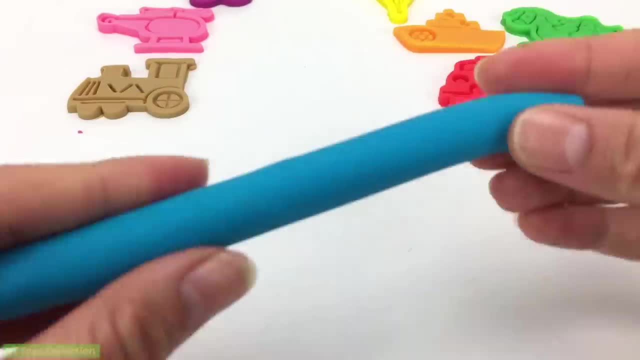 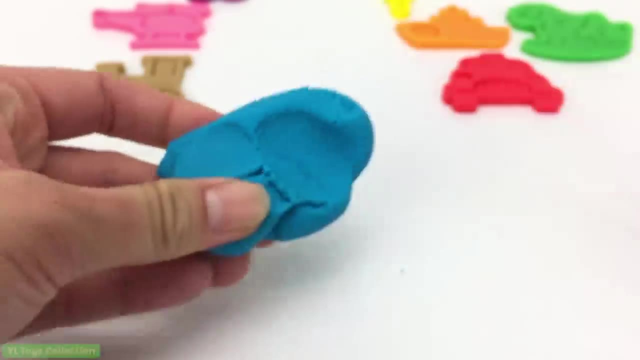 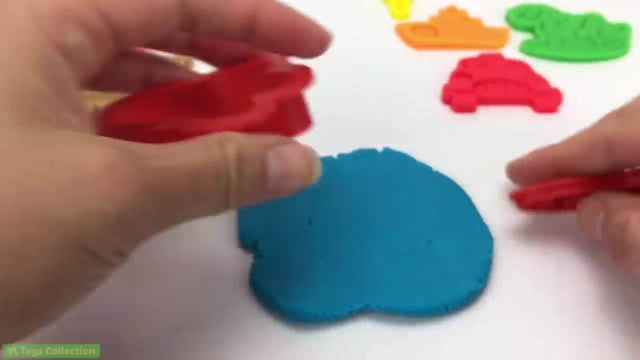 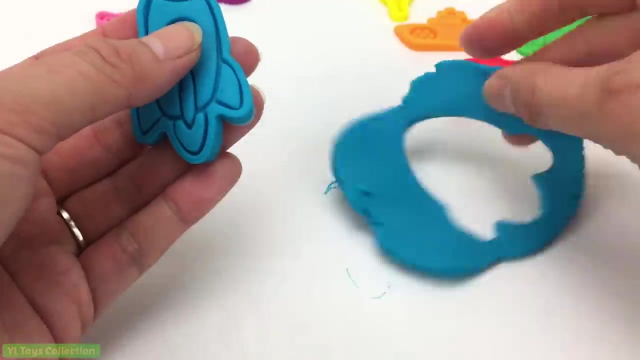 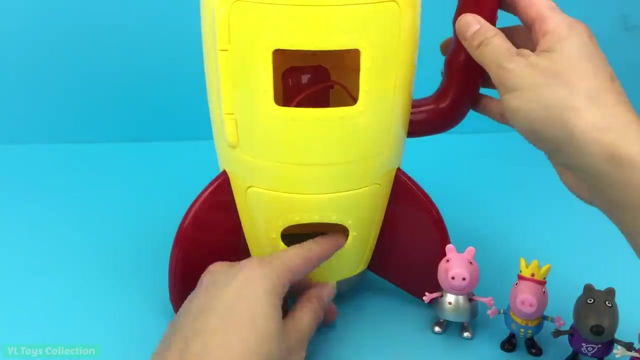 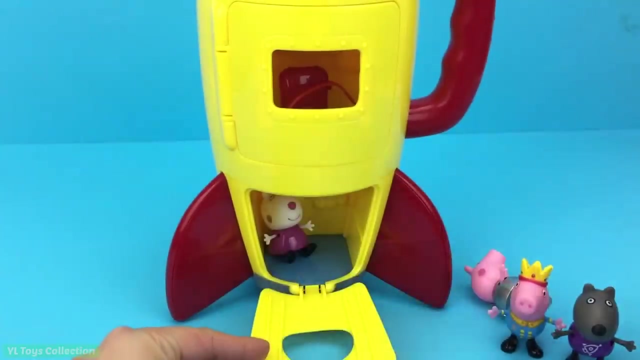 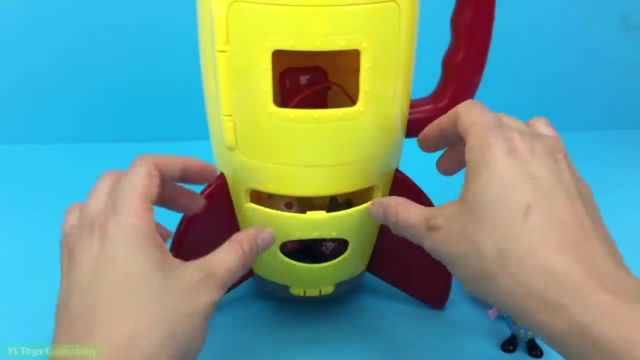 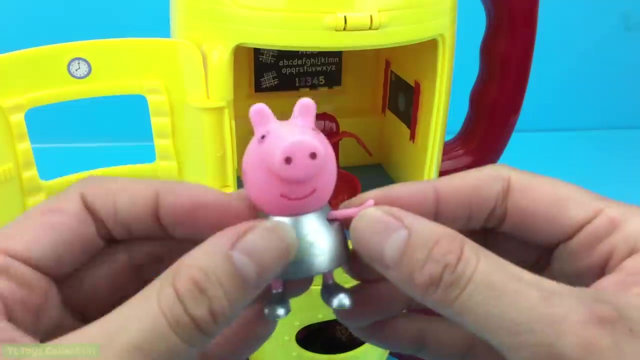 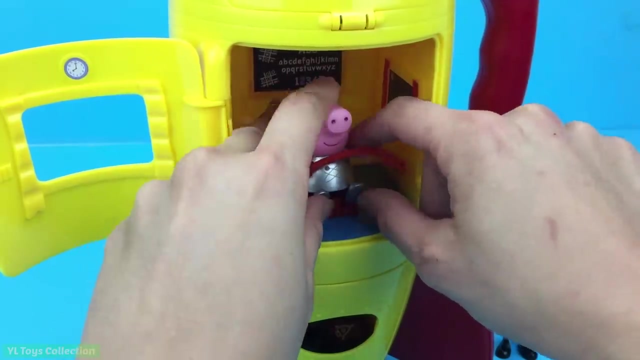 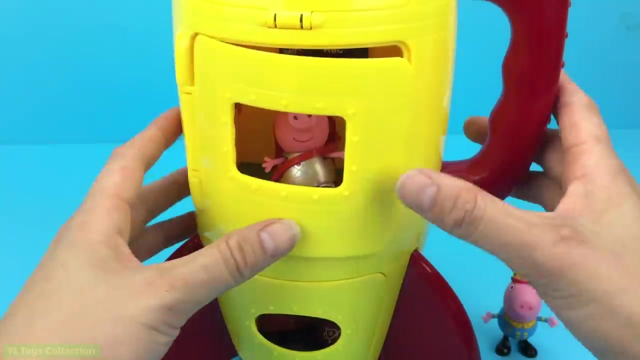 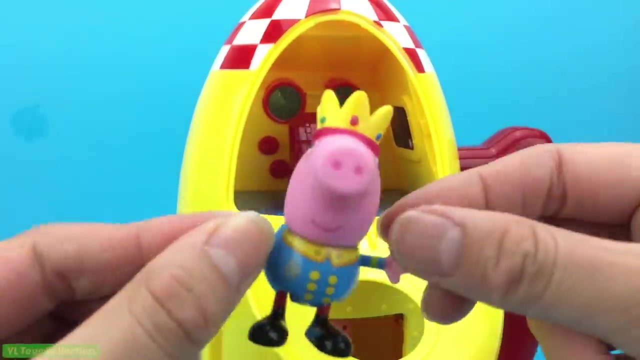 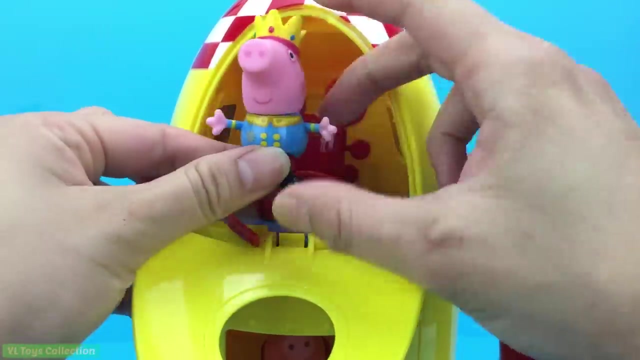 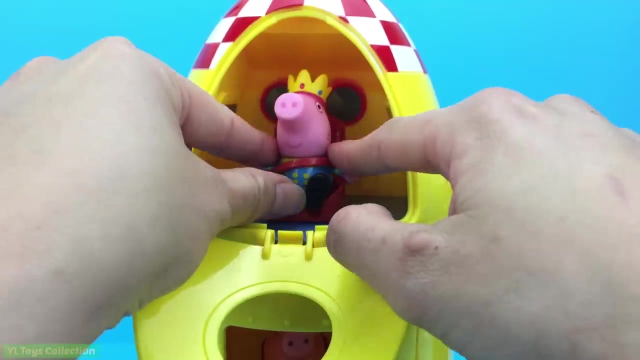 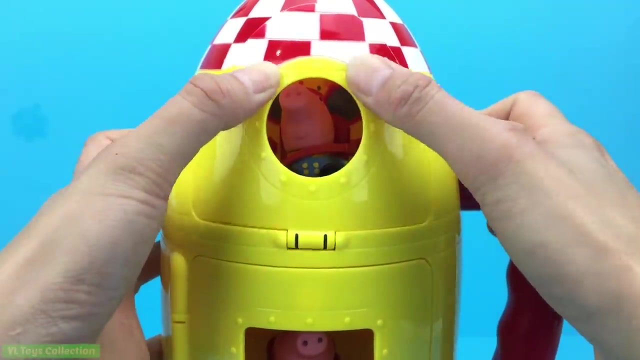 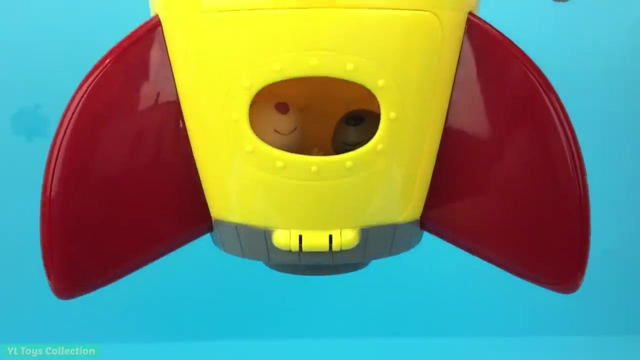 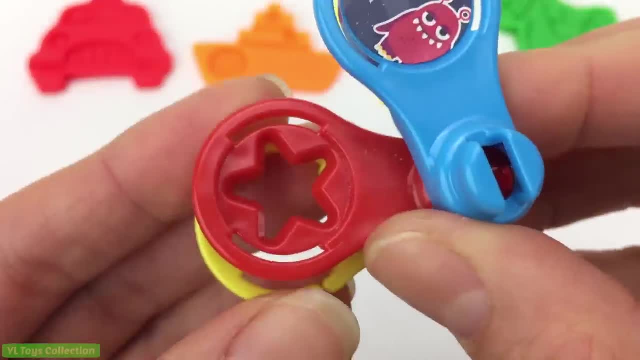 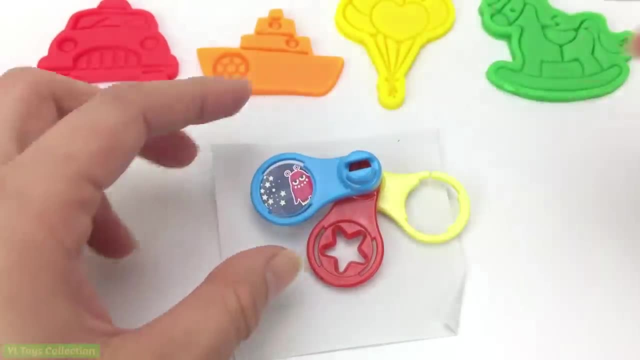 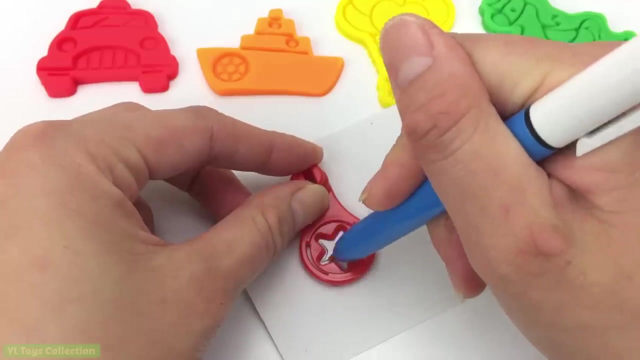 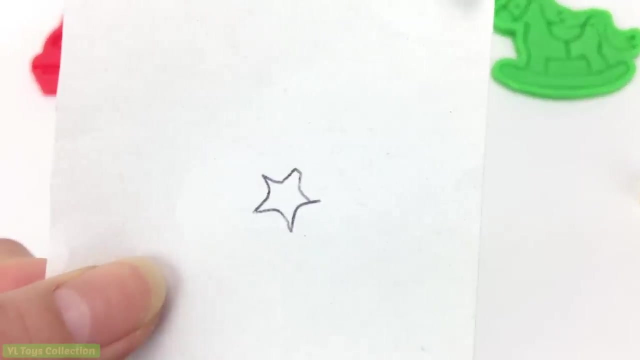 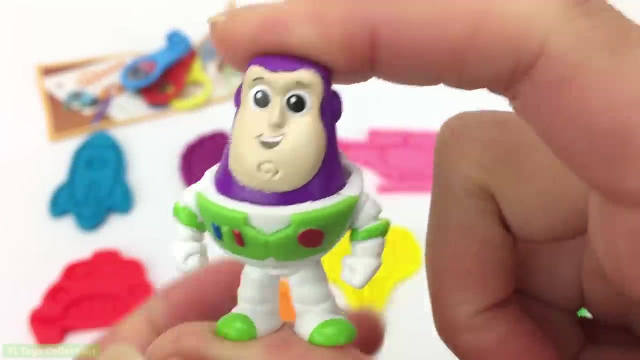 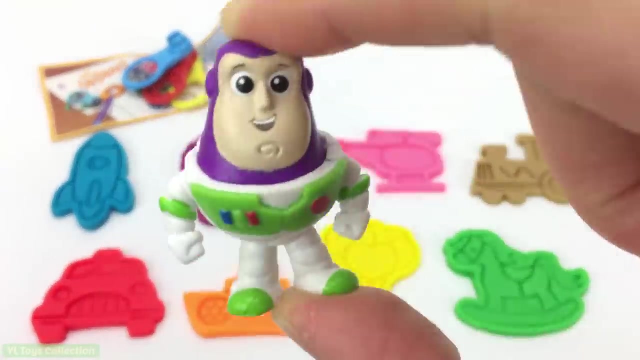 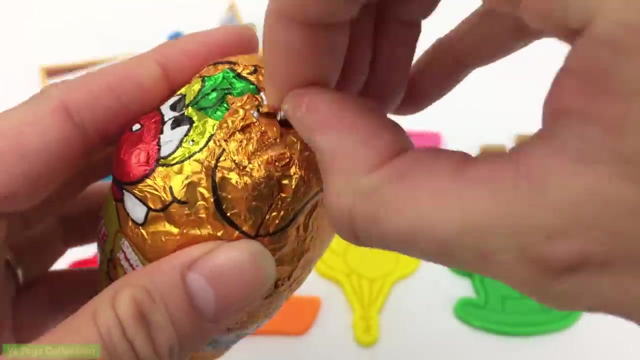 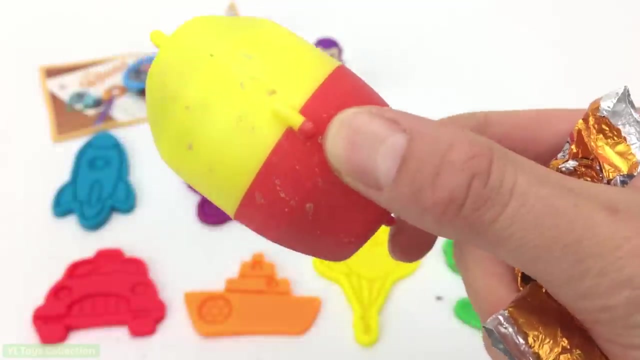 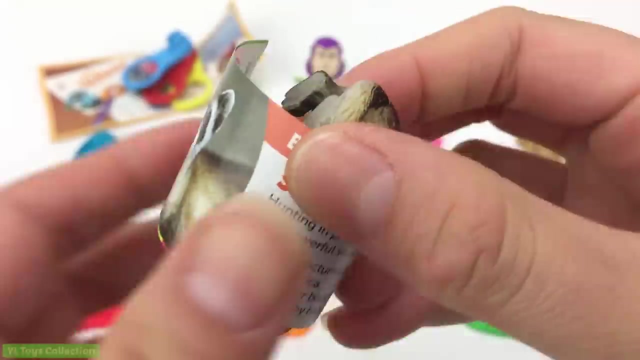 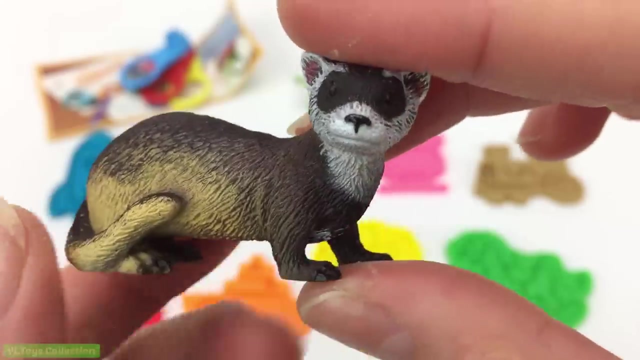 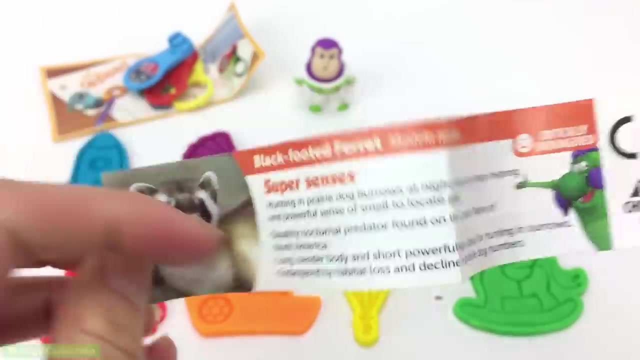 Hooray, Hey Lu Lu. skip to my Lu Lu Lu. skip to my Lu Lu Lu skip to my Lu. skip to my Lu, my darling. Found my partner, love is true. found my partner, love is true. found my partner, love is true. skip to my Lu, my darling.